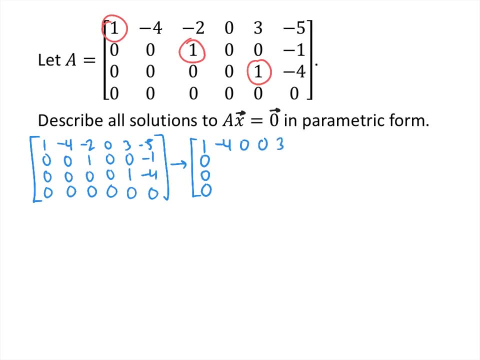 That's going to give us a 0 here and 2 times negative. 1 plus negative 5 is negative 7.. And then row 2 stays the same And row 3 stays the same And row 4 stays the same. 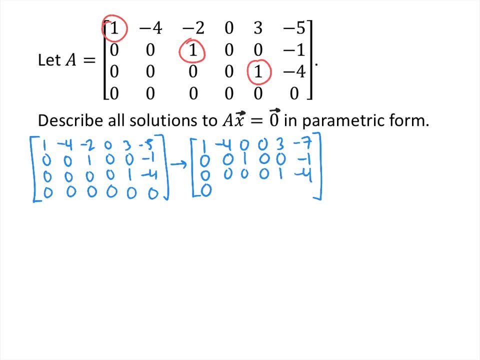 And the rest of the rows all stay the same, And then the last row operation we're going to do is we're going to replace row 1 by negative 3 times row 3.. So that's going to give us a 0 here. 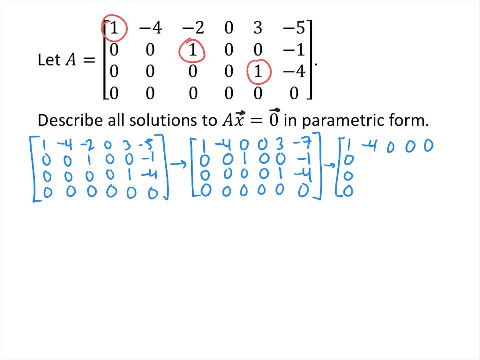 Negative 3 times negative. 4 is positive 12, plus negative, 7 is positive 5.. And now our matrix is in reduced echelon form. So again, our pivots are in columns 1,, 3, and 5.. 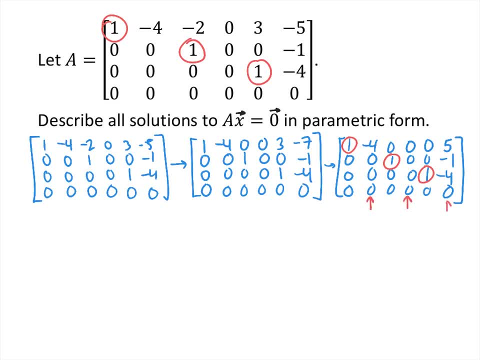 And we've got no pivots in columns 2,, 4, and 6.. Now, remember, we're solving the matrix equation: AX equals 0, where this matrix, this matrix with four rows and six columns, that's A. So this is not an augmented matrix. 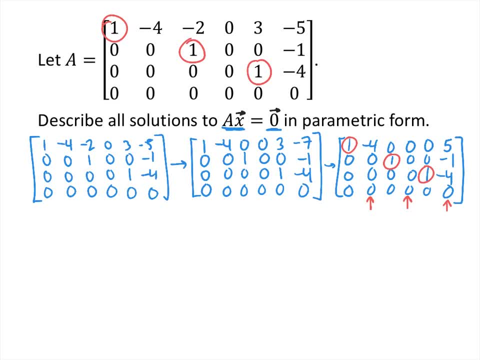 This is the coefficient matrix, And so if we had had an augmented matrix, we could imagine that we have an X and we could have an extra column of 0s here. That extra column of 0s wouldn't have been affected by any of these row operations. 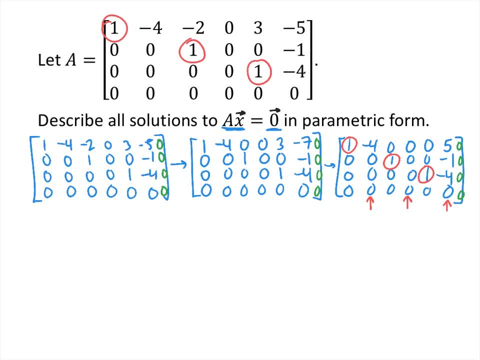 And so, if it helps, we can imagine that we have that extra augmented column of 0s to represent this 0 vector on the right-hand side of our matrix equation. In this case, our general solution has the form: X1 minus 4X2 plus 5X6 equals 0.. 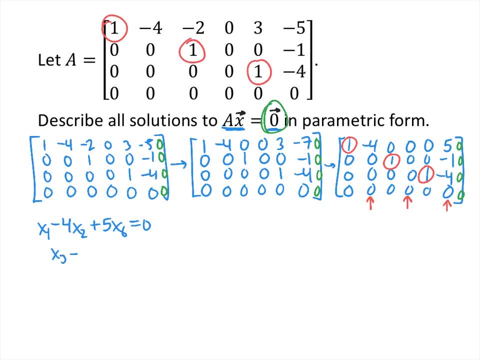 Our second row of our matrix represents the equation X3, minus X6 equals 0.. And the third row of our matrix represents the equation X5 minus 4X6 equals 0.. If we solve that for the basic variables, what we get is X1 equals 4X2 minus 5X6.. 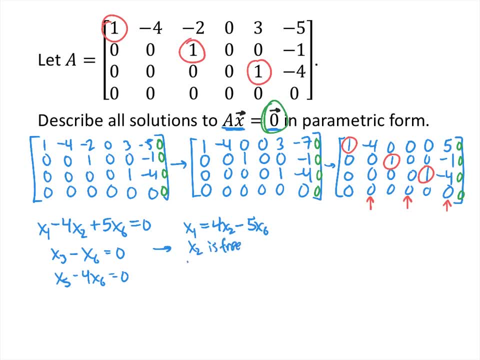 X2 is free because we don't have a pivot in column 2.. X3 equals X6.. X4 is free because we don't have a pivot in column 4.. X5. equals 4x6, and x6 is free because we don't have a pivot in column 6.. 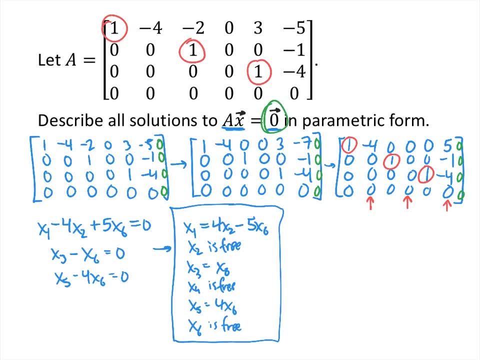 So this right here is the general solution. That's not what the problem is asking us for, but this is sometimes what we want to look at. So this is the general solution of this matrix equation. So if we want the parametric solution, what we want to do is: 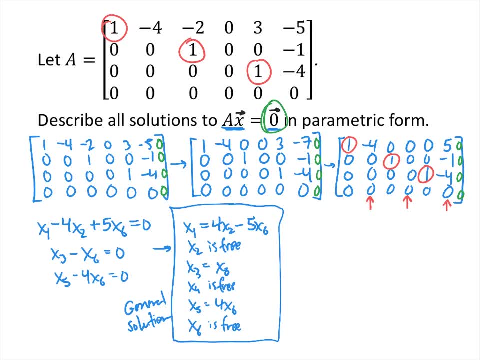 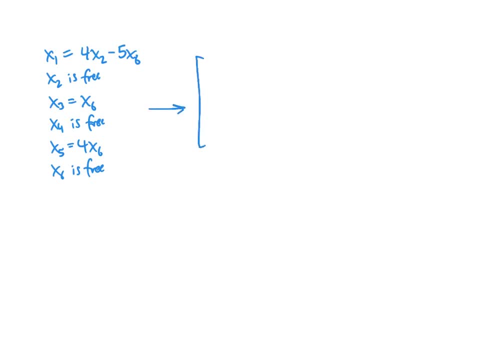 take this general solution and write it in the form of a vector. So here's our general solution. once again and again, what we're hoping for is to write this in the form of a vector. So the vector that we're looking for is what's the vector x that solves that original matrix? 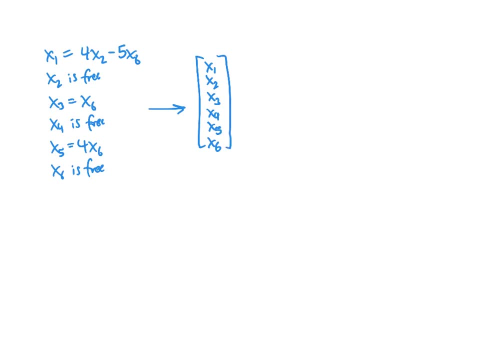 equation. So we know we have six variables, x1 through x6.. What do those variables equal? Well, at first glance we can just look at our general form of our solution and write that in vector form. So we get 4x2 minus 5x6.. x2 just equals itself, x2 just equals x2.. x3 equals x6. 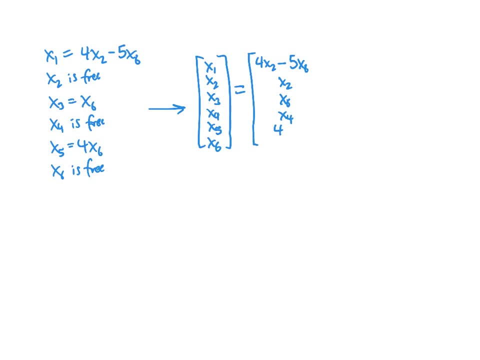 x4 is free, so x4 just equals itself. x5 is 4x6.. And then x6, again is free, so x6 just equals itself. Now to make this a little bit easier to understand, notice that we have three free variables: x2, x4, and x6. 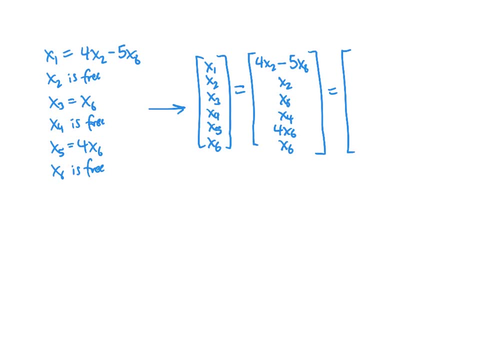 So I'm going to rewrite this so that we arrange it, so that it's easier to see which coefficients are going with which variables. So we've got 4x2, and then I'm going to leave a space where x4 would go if we had any x4s, and then minus 5x6. 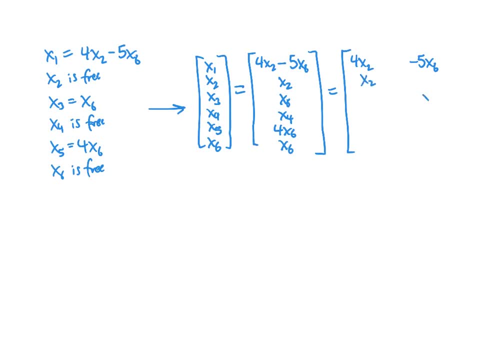 And then next we have just x2.. Next, in the third entry, we just have x6.. In the fourth entry, we just have x4.. In the fifth entry we have 4x6.. And in the sixth entry we have x6. 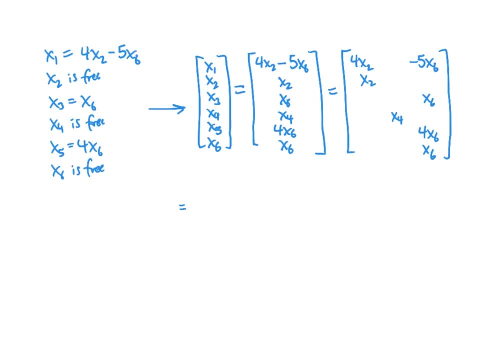 And now I can break this apart according to each of those three free variables, I've got 4x2,, x2, and then 0, 0, 0, 0, because I don't have any x2s in those last four components. 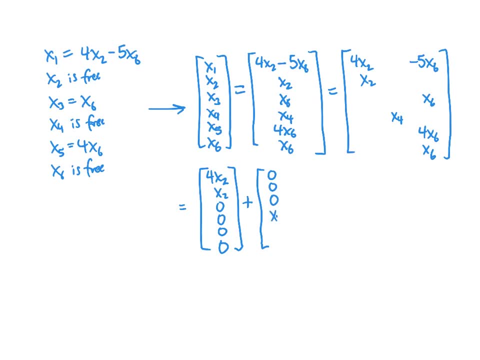 And then for x4, I only have x2, and then I only have a single x4 in the fourth component and then 0s everywhere else. And then for x6, I've got negative 5x6s, then I don't have any x6s and I've got an x6,. 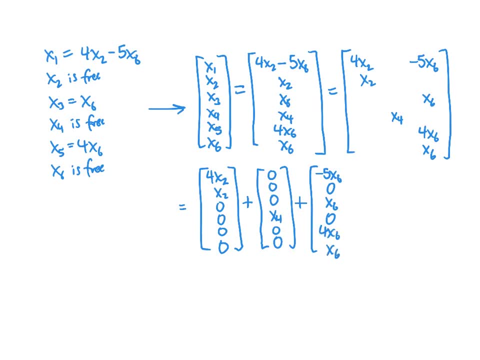 and then again no x6s, 4x6, and then finally x6.. And now we simply pull those scalars x2, x4, and x6, out of each of those vectors, So we get x2 times the vector 4, 1, 0, 0,, 0, 0. 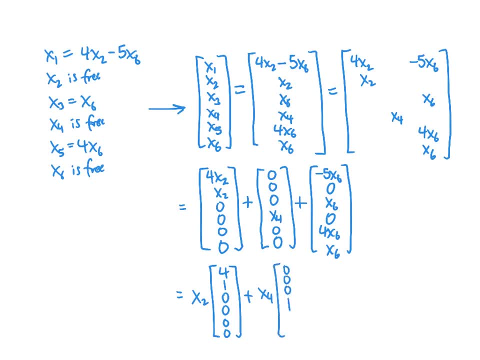 x4 times the vector 0, 0, 0, 1, 0, 0, 0.. 1, 0, 0,. and x6 times the vector negative: 5, 0,, 1, 0,, 4, 1.. 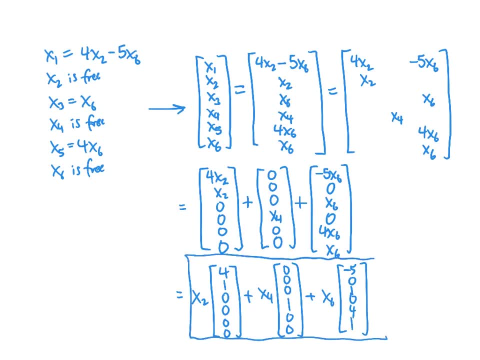 And this is what we're looking for when we say the parametric form of our solution. This is the parametric form. We say that x2,, x4, and x6 are the parameters and that this gives us our parametric form of our solution. 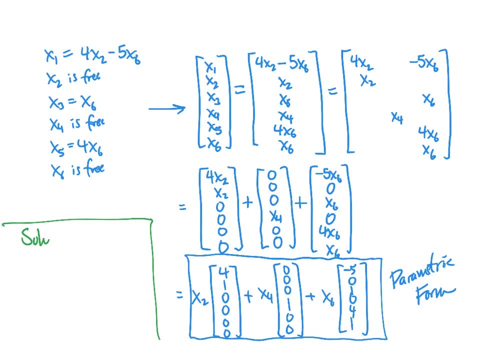 Another way to think about what this is telling us is that the solution set- again not what the question was asking for here, but the solution set- is the span of the three vectors 4, 1, 0, 0, 0, 0,. 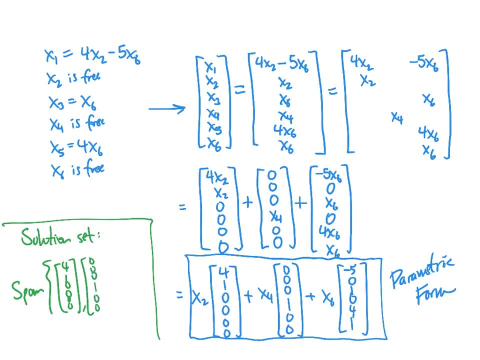 0, 0, 0,, 1, 0, 0, and negative: 5, 0, 1, 0,, 4, 1,, because what span means here is that we are looking at all possible linear combinations. 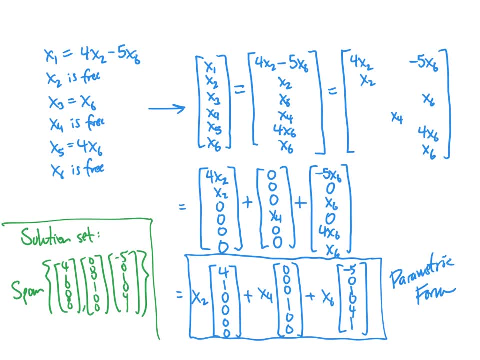 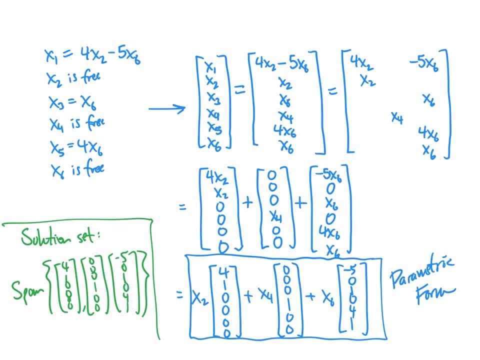 and negative: 5, 0, 1, 0, 4, 1,. anything that's a linear combination of those three vectors will be in the solution set, and that's exactly what we want when we describe the solution set. 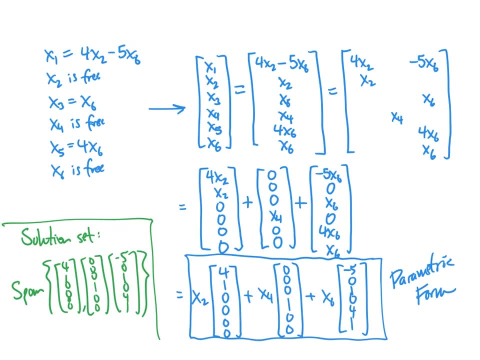 So hopefully this helps explain the difference between the general solution, the parametric form of the solution and the solution set. 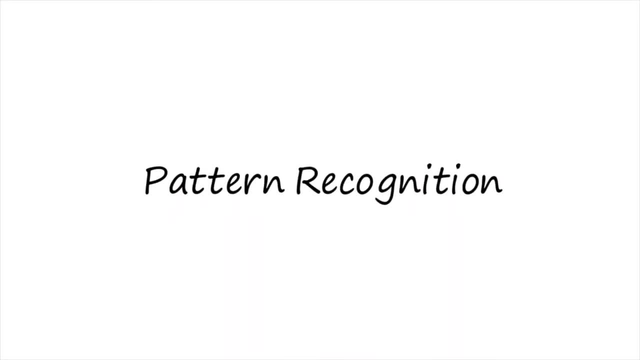 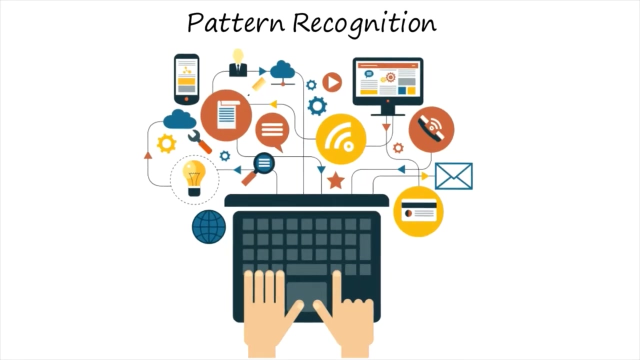 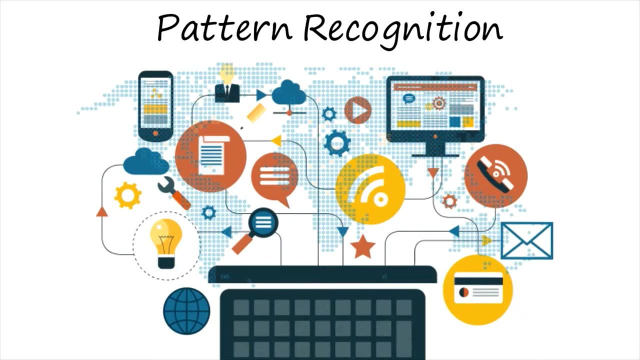 What is pattern recognition? It is a very important concept because this is the base. Everything around in this digital world is the pattern. So nowadays we are surrounded by digital gadgets. So basically, whenever we are talking about digital world, everything around this digital world is considered as pattern. Means a pattern can.